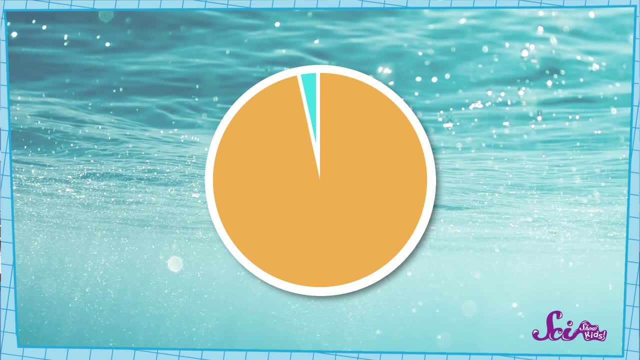 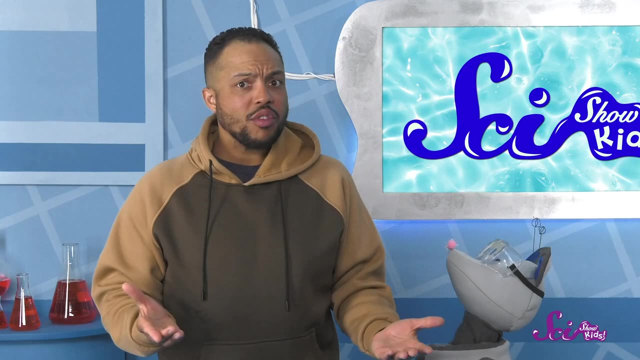 But here's the thing: If we look at our chart again, we can see that only about this much of Earth's water is fresh, Which isn't a lot, And we can't use a lot of Earth's fresh water either. Good question, Squeaks. 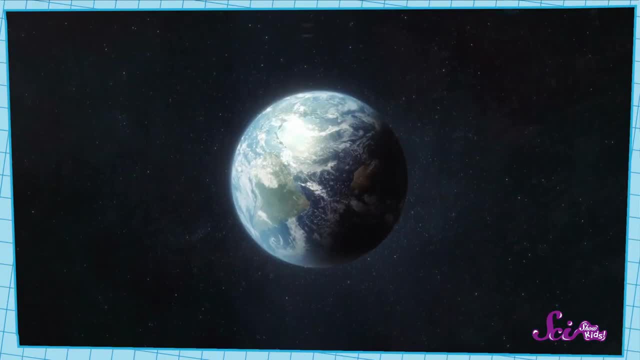 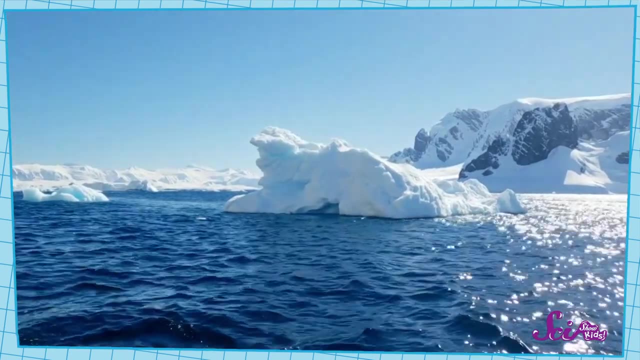 To see why. let's look at the Earth from space again. Most of our planet's fresh water is frozen into ice. A lot of it is at Earth's north and south poles. To use this frozen water, we'd have to get to it, let it melt and take it to where we 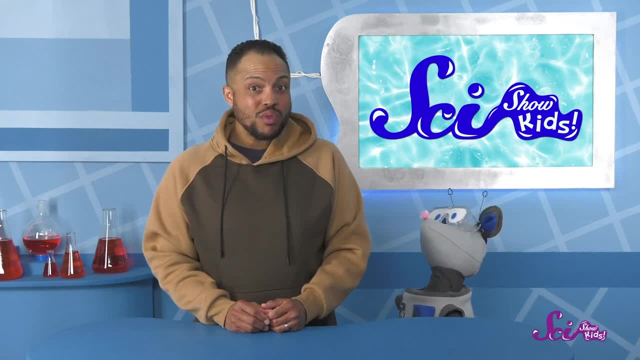 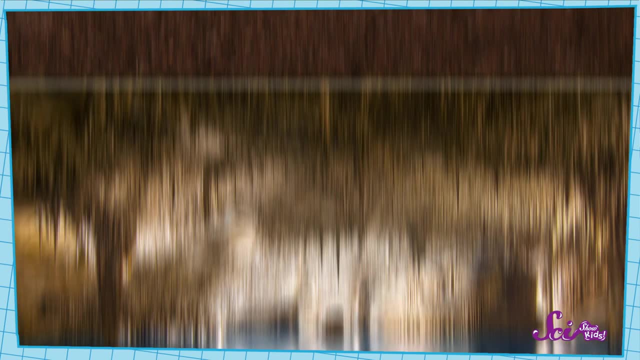 need to use it. That's a lot of work, so this water is really hard to use. Other fresh water is under the ground. We can get to a little of it, but most of it is so deep that we can't access it. 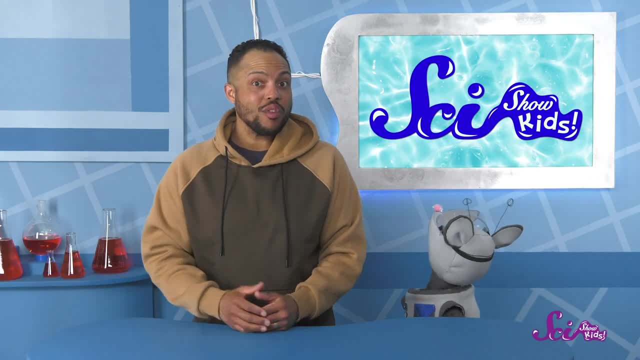 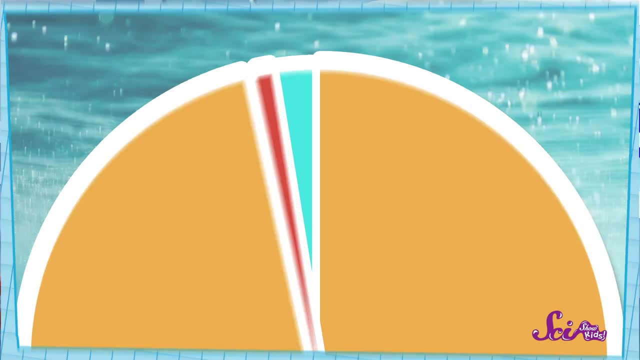 So if we take away the fresh water that's frozen or is in a place where we can't use it, that leaves us with only this much for all of the people on Earth to use, And that's where not wasting water comes in. 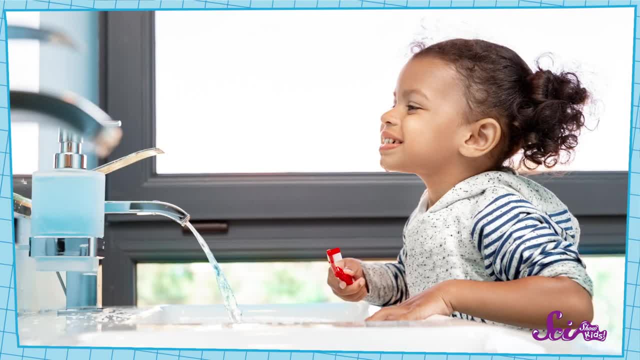 The Earth isn't going to run out of fresh water, Even once you use fresh water. you're not going to run out of fresh water Even once you use fresh water. you're not going to run out of fresh water Even once you use fresh water to brush your teeth or wash your hands. it eventually gets. 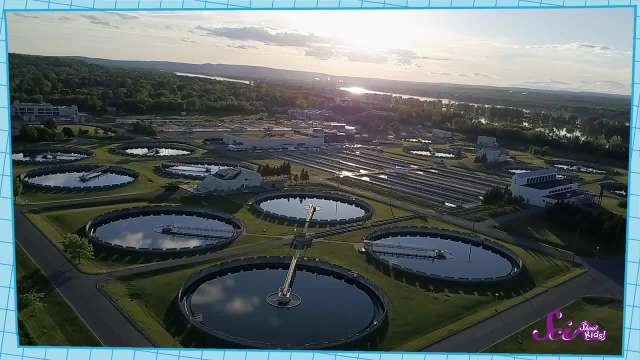 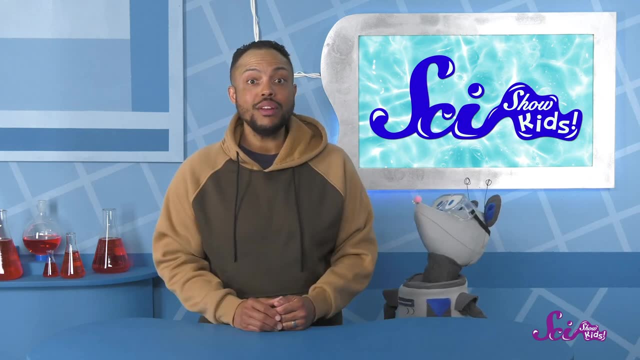 cleaned up at special buildings and put back into the water supply for other people to use, But that process still takes some time, so we need to do our part to make sure there's always enough clean, fresh water for everyone to use every day. 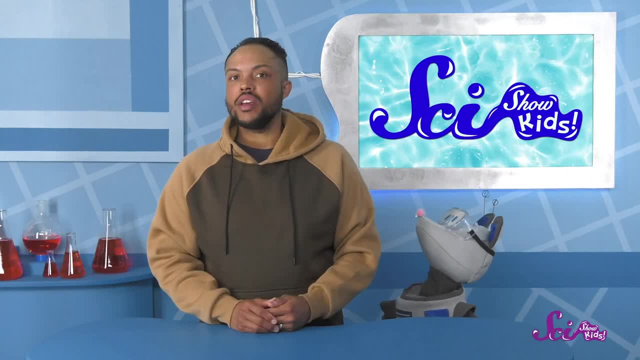 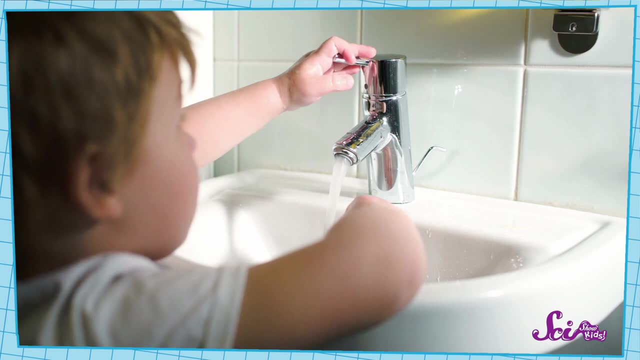 That's a great question. I'll work on fixing the faucet, but there are also some easy things you can do to help. Probably the easiest thing to do is to make sure that you turn off the faucet all the way when you're done using it. 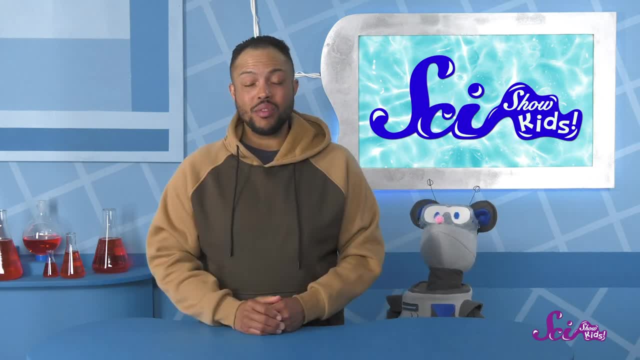 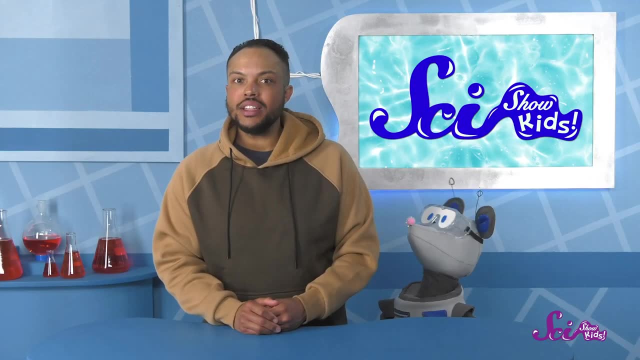 Even a little bit of dripping can add up to a lot of wasted water. Another easy thing: You can turn off the tap while you brush your teeth. Just by doing this you can save about 30 liters of water a day. That's almost 8 big jugs of milk. 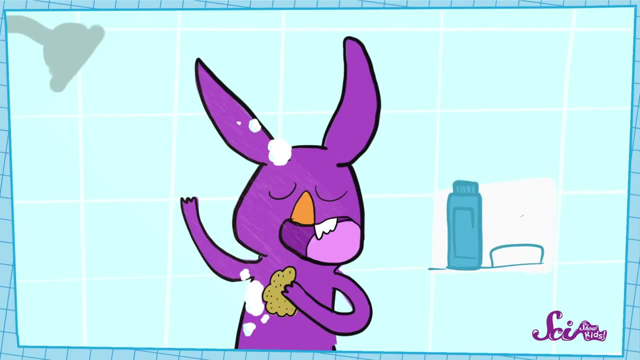 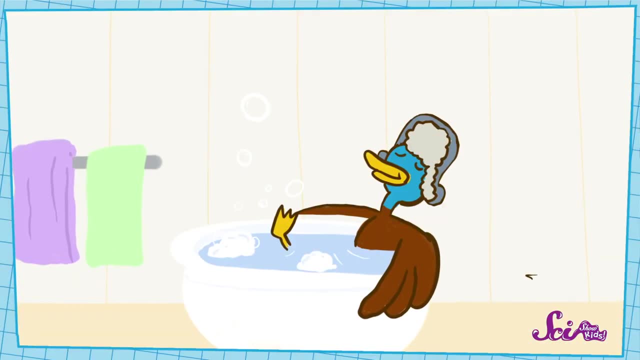 There are also things you can do to save water when it's time to get clean, too, Like taking a shorter shower can help See if you can take one in less than 5 minutes as long as you're still washing up, Or if you'd like baths instead, you can use the bathtub stopper right when you take a shower.